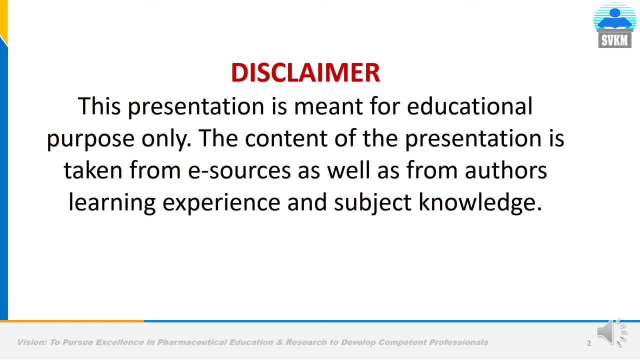 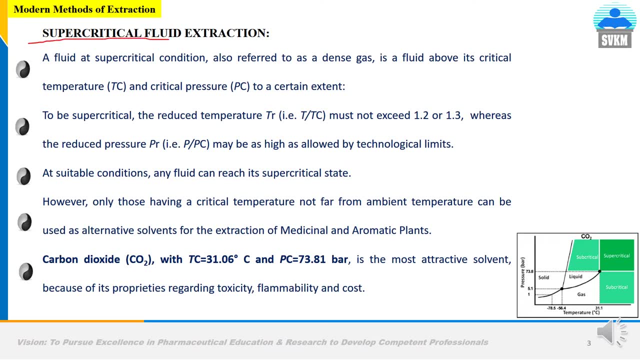 Explemer. this presentation is meant for educational purpose only. The content of the presentation is taken from e-sources as well as from author's learning experience and subject knowledge. Dear students, the supercritical food extraction technique is one of the unique techniques of extraction of active constituents from the drug material wherein the gas is utilized as a solvent. 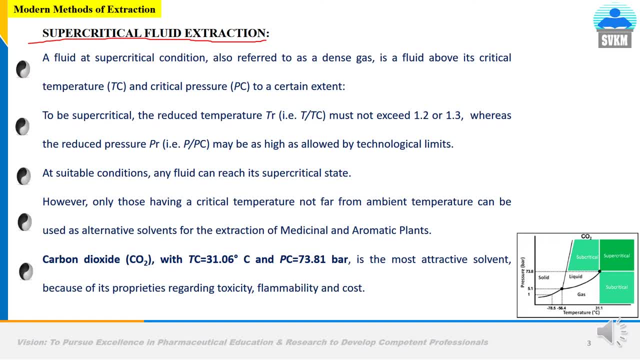 How These gas are converted into a solvent or into a liquid by applying increased pressure and decrease in temperature. so the temperature is decreased and pressure is increased. So at this point or at this point or at these factors, any gas can get converted into liquid. 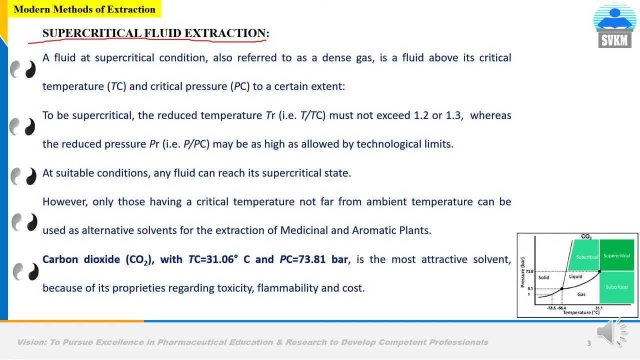 and then that liquefied gas can be used as a solvent. So we need to first understand what is this conditioning. End is where the gas converts into liquid, so that point is called as supercritical point, wherein gas can easily get converted into a liquid form, so a fluid, at supercritical condition. 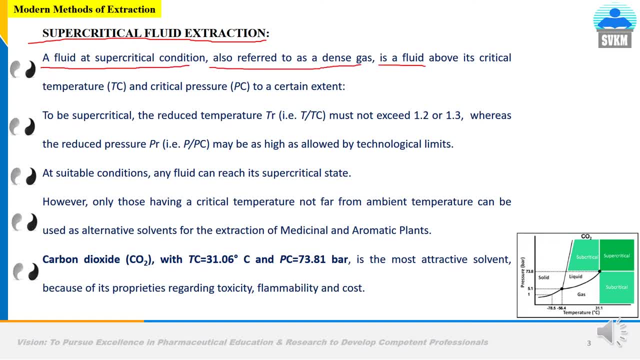 also referred to as a dense gas, is a fluid above its critical temperature and critical pressure to a certain extent. that extent is nothing but to be supercritical. the reduced temperature, so the temperature should be reduced, that is, in minus and must not exceed to 1.2 or 1.3 degree, whereas 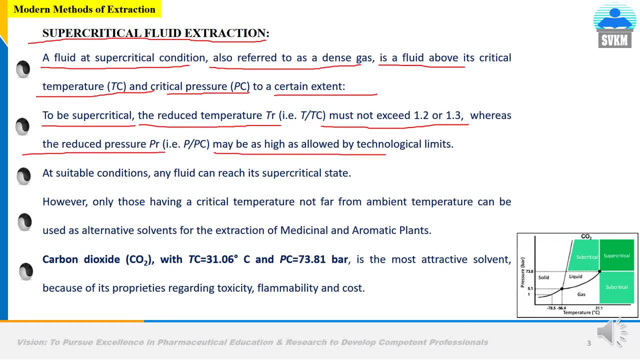 the reduced pressure may be high, as allowed by technological limits, which means here the gas is pressurized- okay, above its normal level and the temperature is reduced, and because of this condition the gas attains a supercritical point, where the gas converts into any fluid or liquid and thus at suitable condition. 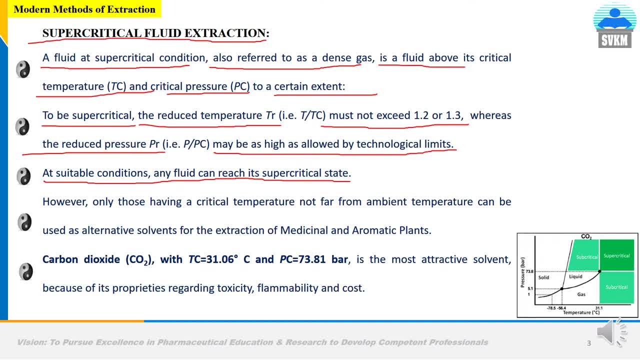 any fluid can reach its supercritical state. however, only those having critical temperature not far from ambient temperature can be used as alternative. solvent for extraction of medicinal and aromatic plants means there are certain limited gas which can be converted into liquid by applying a set pressure and by reducing the temperature. 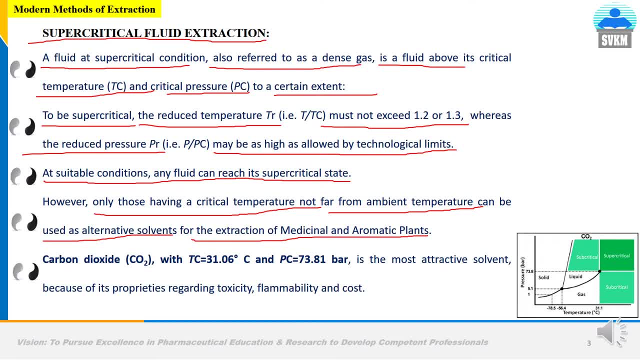 so that it can get converted into fluid and can be used as a appropriate solvent for the extraction of various phytoconstituents from the medicinal and aromatic plants. and now why this method is only utilized? because there are some thermo-liable phytoconstituents which get degraded at high. 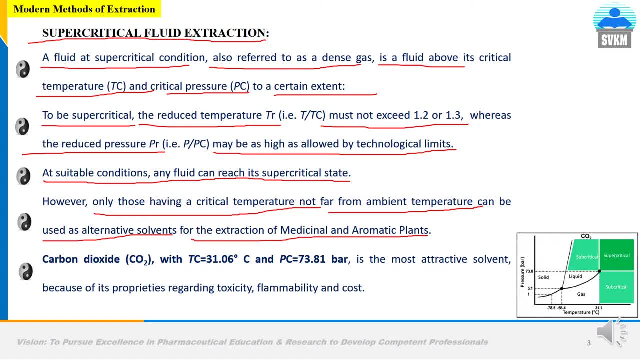 temperature. this technique has the beauty that where this gas is converted into liquid at very less temperature and because of this this solvent is not going to hamper or not going to alter a physical chemical properties of the phytoconstituents, okay, and therefore this technique is one of the unique. 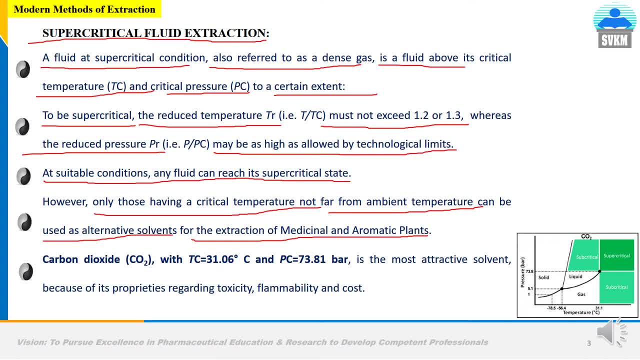 technique of extraction of various array of phytoconstituents. carbon dioxide is a suitable gas so far, which has been studied, reported and documented with the temperature 31.06 degree celsius and pressure at 73.81 bar. is the most attractive solvent because of its properties regarding. 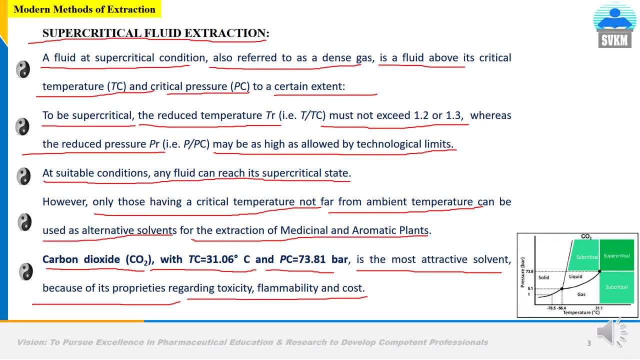 toxicity, flammability and the cost. so cost-wise it is very easy to have easily available, economic, non-combustible, non-toxic, non-inflammable, and therefore this can be. this carbon dioxide can be easily used as a gas, but at super critical point it can be converted into a required solvent to for for the process of. 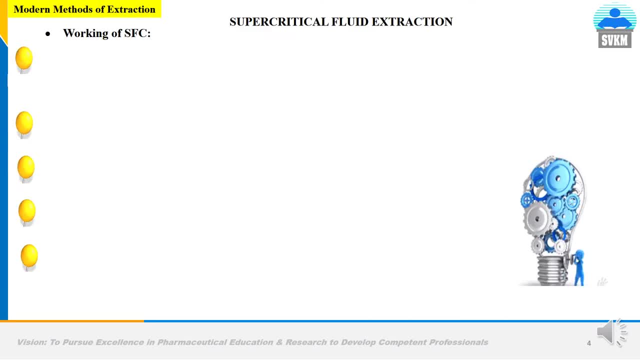 extraction working of supercritical food extraction. the system must contain a pump for the carbon dioxide to pass, a pressure cell to contain the sample, a means of maintaining pressure in the system and a current system so that the pressure of the cell can be created in the system. 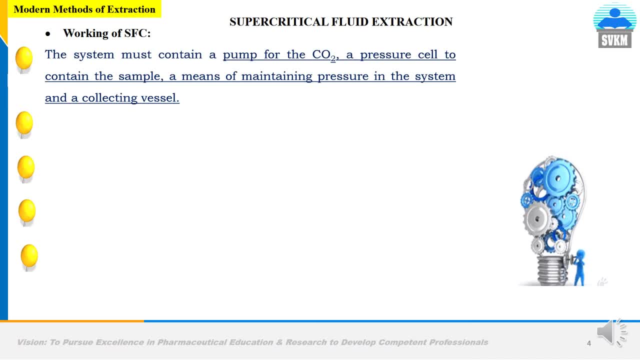 all the way to a very high temperature and the same way the concentration of carbon dioxide as a collecting vessel. So supercritical fluid extraction is designed in such a way that there is a pumping system- wall pumping system- attached at every junction where it first pumps. 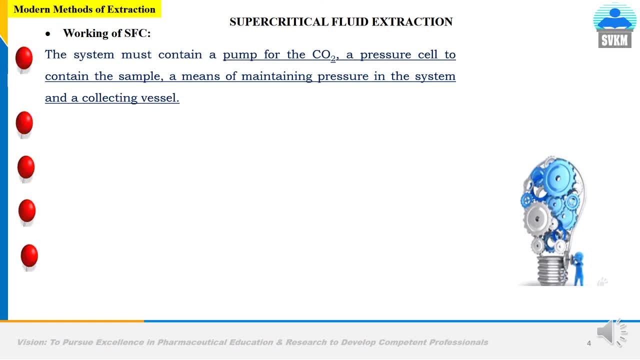 the gas into a, through a wall, through a pump, at a particular pressure and the temperature, so that it can convert into a appropriate solvent by attaining its supercritical point. and then this solvent goes in the extracting chamber where the drug is placed, and then the mixture is takes place. 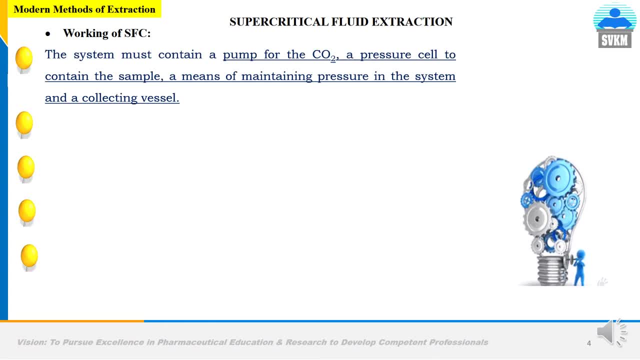 the extraction is takes place and the whole liquid and the extract dissolved active constituent is passes with the same pressure to the columns, to the separators wherein we can separate the phytoconstituent together. Second, the liquid is pumped to a heating zone where it is heated to. 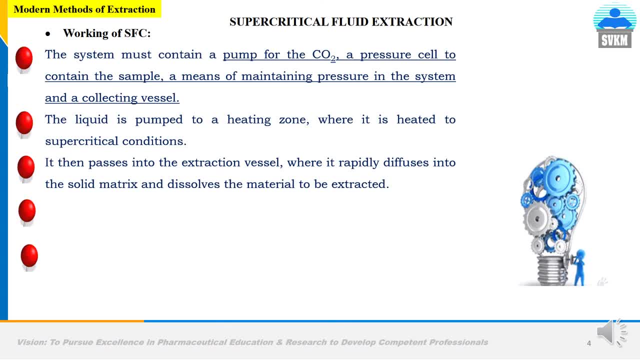 supercritical condition It is then passes into the extractor In the extraction vessel, where it rapidly diffuses into the solid matrix and dissolve the material to be extracted from the crude drug. The dissolved material is swept from the extraction cell into a separator at very low pressure and the extracted material settles down, whereas the liquid converts. 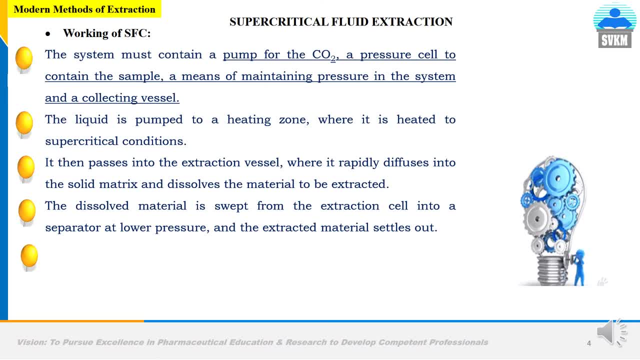 into or get evaporated into gas and again it is reused. the same carbon dioxide gases then further reused. The carbon dioxide can then be cooled and re compressed and recycled for discharge to the water before it gets in to the earnynth atmosphere which round out the seed. 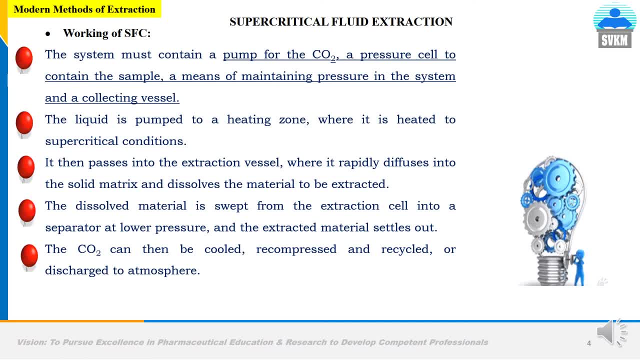 So than in this approach, we will proceed in a highly програмmatic operation of the carbon dioxide, which will be eliminated through the process. In the end it is again recycled and again re pumped into the fish tank, where it can again convert it into a suitable economical product. 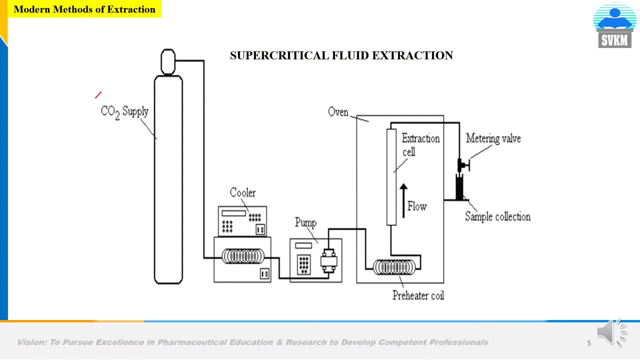 In the working quality of home. justification we can see here, dear student. the carbon dioxide has Cow cost six times the lower volatile members of the blood. Salicylic AcidTA2 are supplied here here and here it gets. carry it, Sergeant ven here. okay, so it's a gas cylinder where this is the pressure wall, so through. 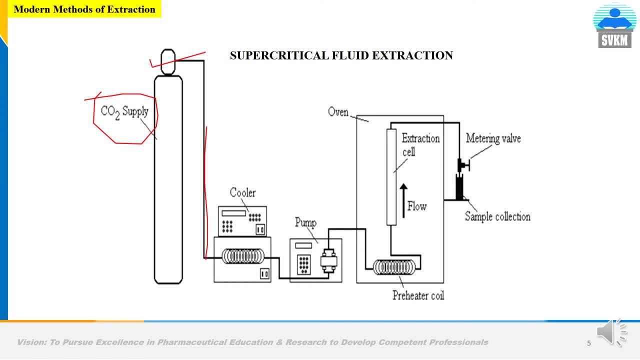 this pressure wall, the gas is supplied in such a way that it get convert, it is compressed and then here the gas is converted into liquid, which is then further pumped- okay, through the channels, through the walls of pumping system, and then it is further brought in the extractor. this extractor is nothing but. 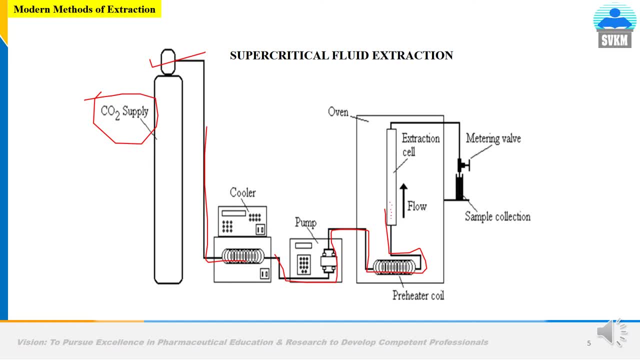 where in the drugs is present, crude drug is present, and then the solvent carbon dioxide is come in contact with the drug for the same period of time and then, after complete extraction, the mixture of the dissolved drug material and the liquid carbon dioxide passes from the extracting chamber to the metering wall. 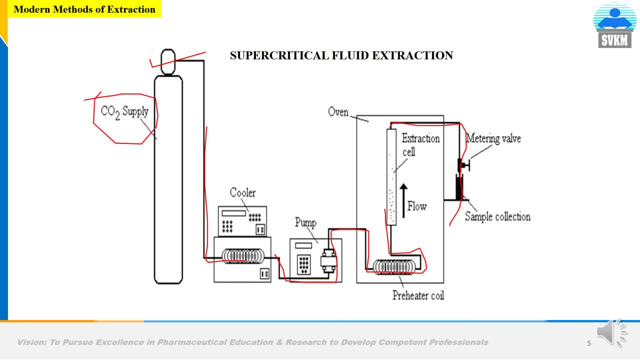 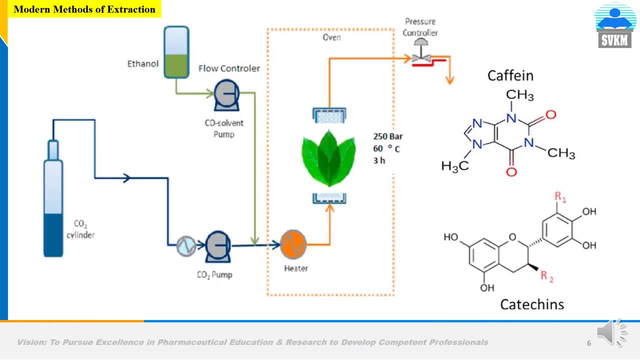 where the liquid carbon dioxide is coming out of the extraction chamber to the metering wall, where the sample is separated and at the same time the liquid gas is further evaporated to convert into gas and which is reused for the further process of extract. method of extraction. method of extraction. so here I have schematically represented the 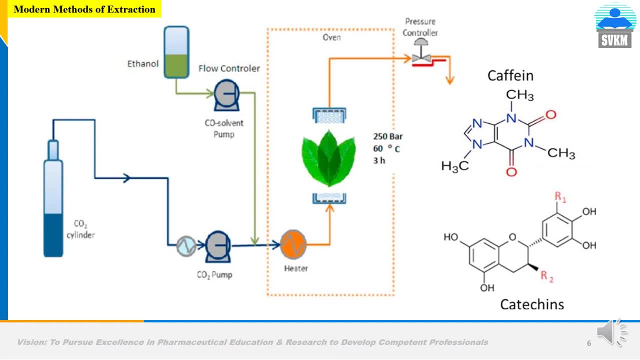 extraction of caffeine and catechin through supercritical fluid extraction. carbon dioxide cylinder is placed in the extraction chamber and then the liquid here which is again passes through the carbon dioxide pump and then it goes. even the solvent also comes here through this chamber. there is a mixture takes. 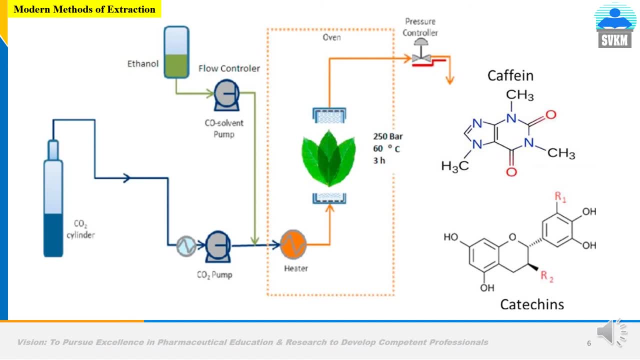 place of the drug. so in the extractor the proper temperature is maintained and then the liquid is extracted further so that you can get the caffeine and catechin together from the tea leaves. so isn't it a beautiful method of extraction of phyto constant? yes, it is, it is. 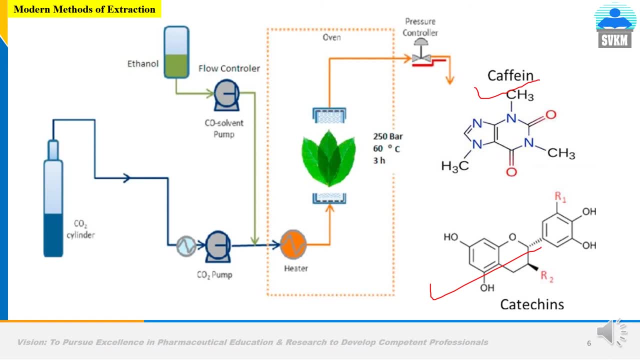 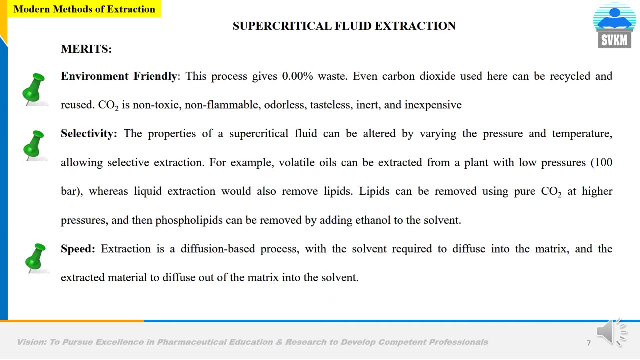 indeed it is okay. so it's a only make use of a carbon dioxide gas into a solvent without hampering the phyto constant merits: environment friendly. this technique is very much environment friendly, so 0.00% waste- even carbon dioxide used here- can be recycled and reused. carbon dioxide is 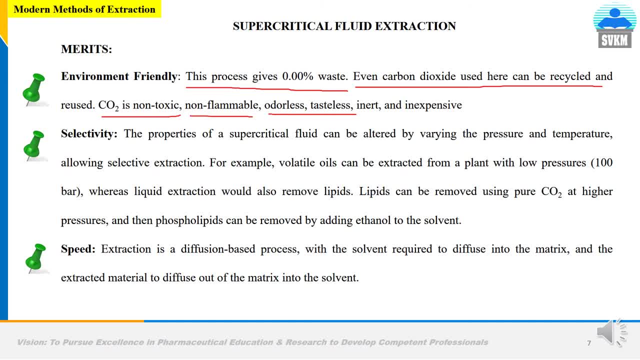 completely non-toxic, non-flammable, easily available, tasteless, inert and very inexpensive. technique, or say inexpensive gas selectivity: the properties of supercritical fluid can be altered by varying pressure and temperature, allowing selectives extraction. it means what? if you want to extract volatile oils, you can increase or decrease the pressure of carbon dioxide. thereby you can make ease. 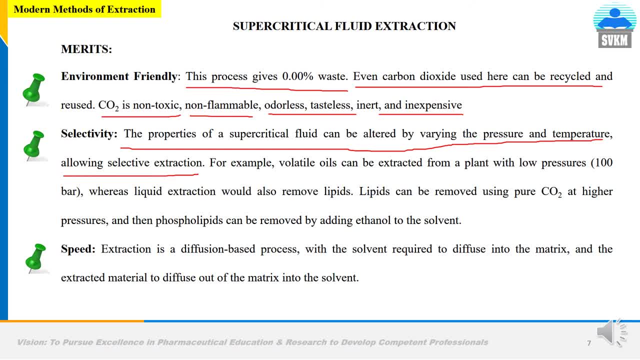 of extraction of that particular phyto constant from the given drug, whereas for liquid extraction would also remove lipids. lipids can be removed by using pure carbon dioxide at higher pressure, and then phospholipids can be removed by adding ethanol to the liquid extractor. so this is 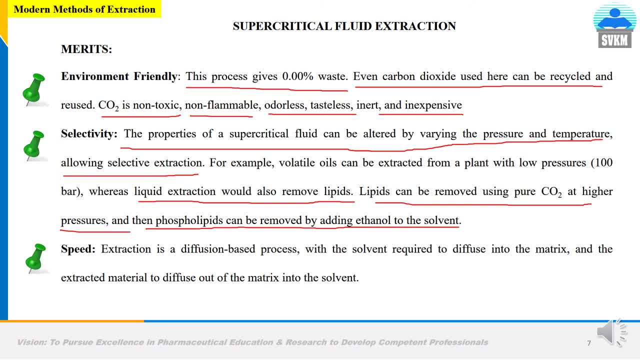 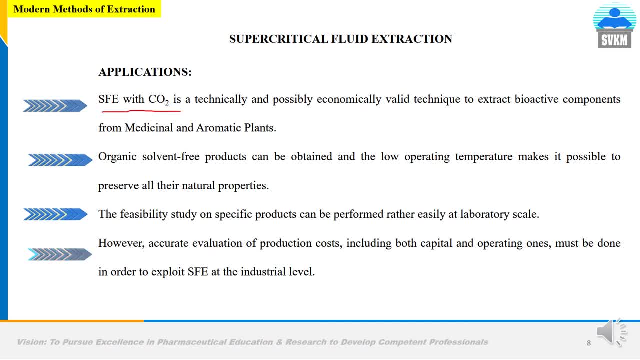 supercritical. food extraction with carbon dioxide is technically and possibly economically valid technique to extract various bioactive components from the carbon dioxide and the phyto constant from the carbon dioxide. to extract the phyto constant from the carbon dioxide to the phyto constant from the carbon dioxide. to extract the phyto constant from the carbon. 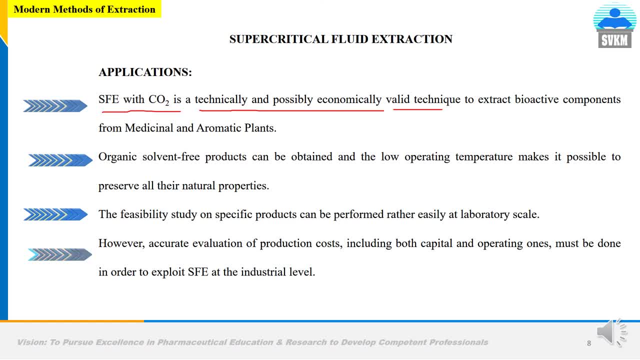 dioxide to extract the phyto constant from the carbon dioxide components from medicinal and aromatic plants of commercial utility, all the constituents which has huge global market and that can be, and that too in its pure form, and therefore the supplier can provide the same phyto constant at the very less rate with the good quality. 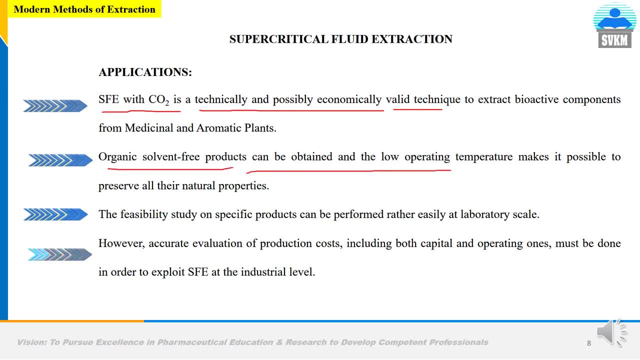 organic solvent free products and can be obtained, and the low operating temperature makes it possible to pressure or to preserve all the natural properties. so, due to this, we are not using any organic solvent. we are simply using carbon dioxide gas in its liquid form, and because of that it is maintaining the complete physicochemical properties of the active constituents. 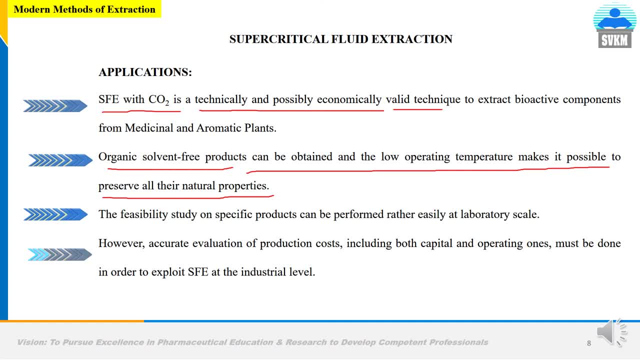 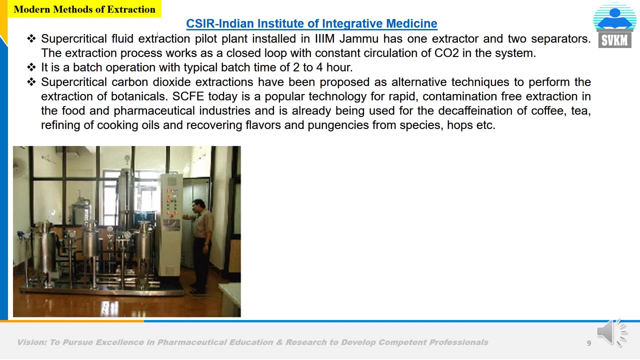 as well as its stability. the feasibility. the feasibility study on specific products can be performed rather easily at laboratory scale and, however, accurate evaluation of production cost, including both capital and operating ones, must be done in order to exploit supercritical fluid at industrial level as well. dear student, this is the example which i have quoted here from: 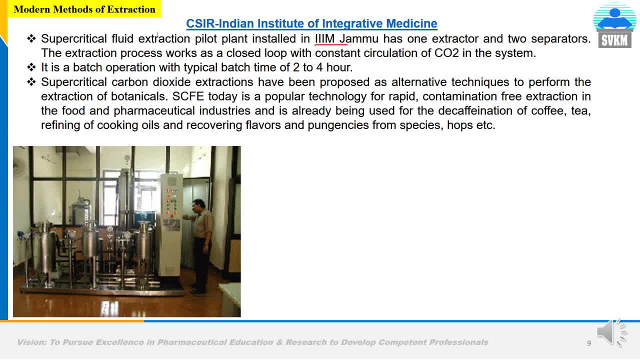 triple i institute of integrative medicine, jammu. they have this system called a supercritical extraction pilot plant installed and there are the two separators, one extractor, in their process. so we can get outsourced from this and this is a batch operation. you can get outsourced from this and this is a batch operation. 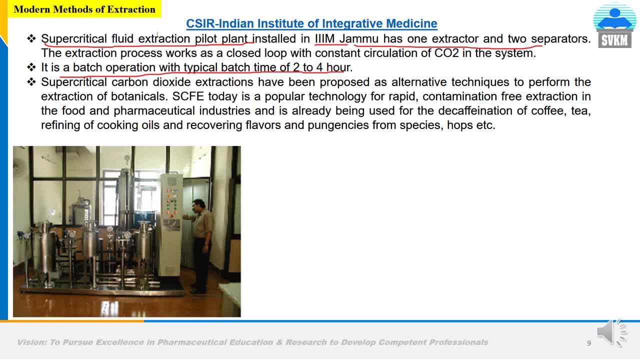 with typical batch time of two to four hours. so in two to four hours the person, the scientist, is standing over there. this is a whole uh component of supercritical fluid extraction that you can see here, which is available in csir, in indian institute of integrative medicine, which provides so many extraction, isolation, purification. 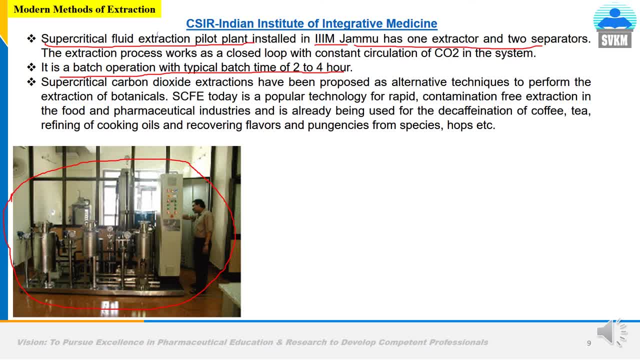